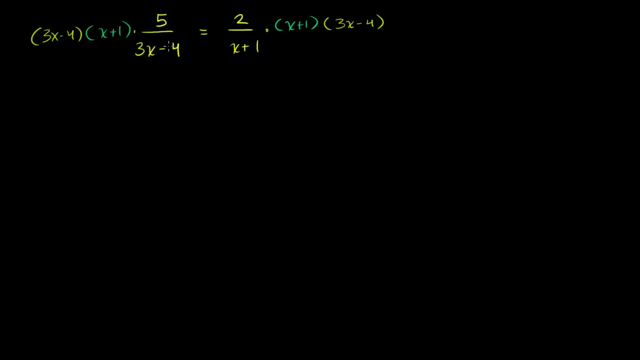 So I'm just multiplying both sides of this equation, times this and times this. Whatever I multiply on this side, I also have to do on this side. Now, what is it going to simplify to? Well, this 3x minus 4 is going to cancel out with this 3x minus. 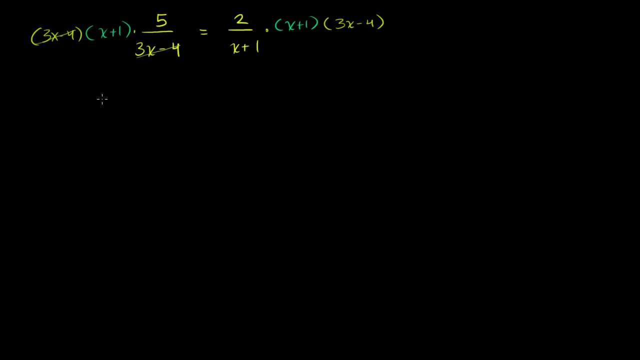 4.. So the left-hand side is just going to be x plus 1 times 5. Or 5 times x plus 1.. And my right-hand side, this x plus 1, is going to cancel with that x plus 1.. 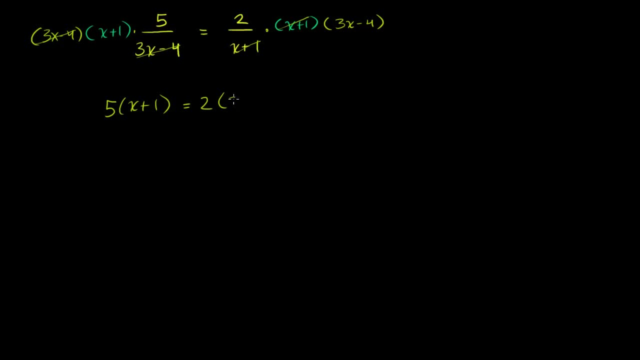 It's just going to be equal to 2 times 3x minus 4.. 2 times 3x minus 4.. And if you just look at it, if you didn't look at what we actually did, it looks like we did something called cross. 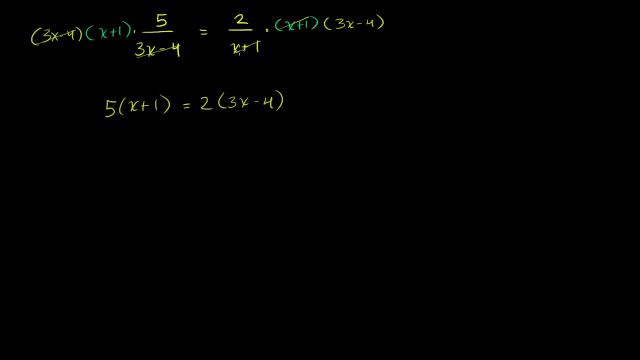 multiplying When you have something over something is equal to something else over something else. notice: The end product when we multiplied both sides by both of these expressions was 2 times 3x minus 4 is equal to 5 times x plus 1.. 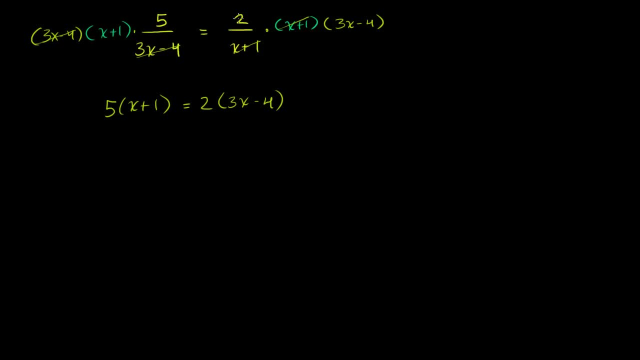 So it looks like we cross, multiplied 5 times x plus 1, is equal to 2 times 3x minus 4.. But the reality is we didn't do anything new. We just multiplied both sides by this expression and that expression. 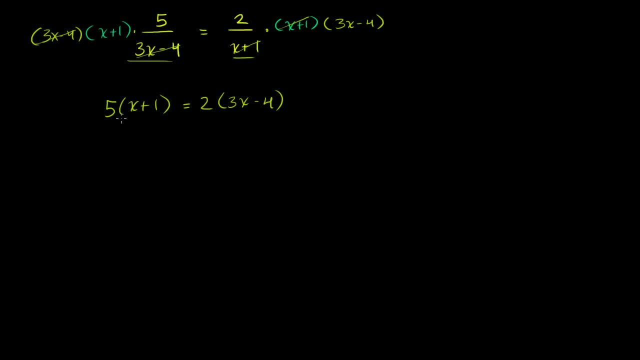 But now we just have a straight-up linear equation. We can just simplify and solve. So the left-hand side becomes 5x plus 1.. That's it Plus 5.. Just distribute the. 5. Is equal to 6x minus 8.. 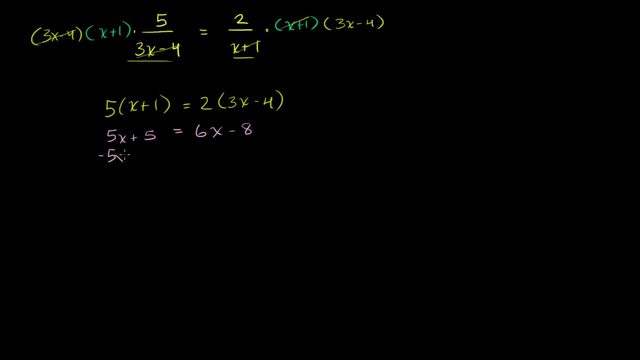 Now we could, let's say, we subtract 5x from both sides. If we subtract 5x from both sides, the left-hand side just becomes a 5. The right-hand side. we are left with x minus 8. And now we could add 8 to both sides. 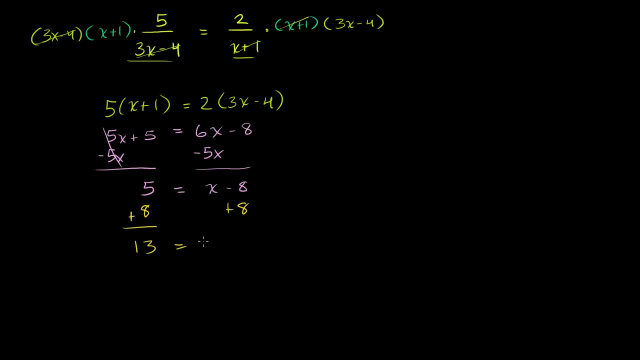 The left-hand side Comes 13.. The right-hand side is just an x And we're done. x is equal to 13.. Solves this equation. You could even try it out: 5 over 3 times 13 is 39.. 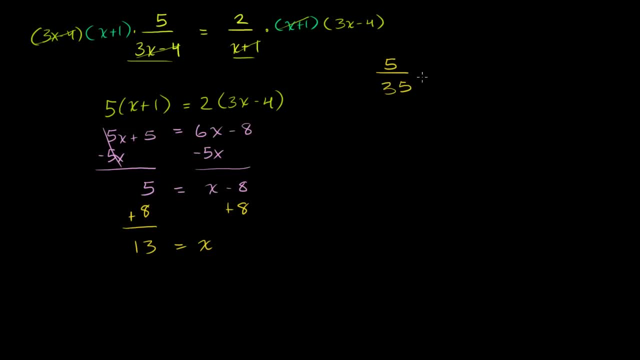 39 minus 4 is 35. And this should be equal to 2 over 13 plus 1, or 14. And they both equal 1. seventh, So it checks out: Let's do a more, Let's do a more involved one. 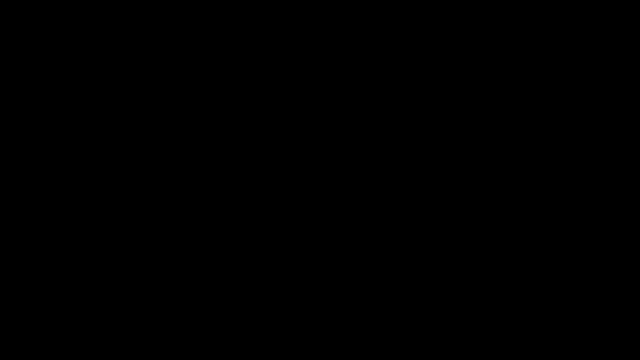 Let's do a more involved problem. So let's say I had this was pretty involved right here. Let's say I have negative x over x minus 2 plus- I'm going to give it some space here- 3x minus 1 over x plus 4. 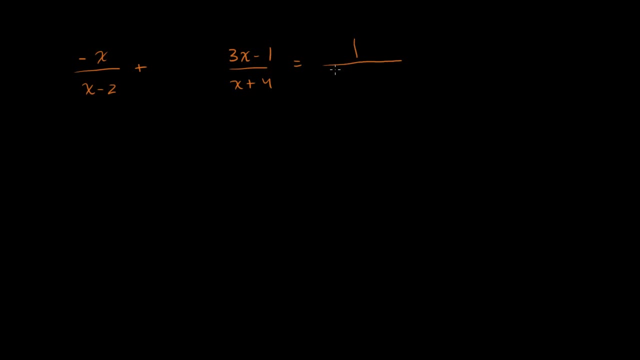 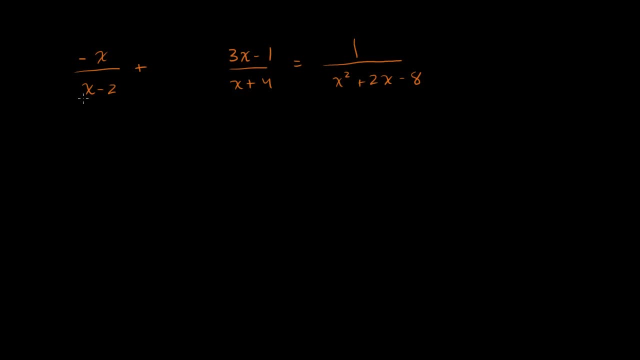 by the least common multiple of this expression, this expression and this expression. But this one looks like it can be factored, So maybe it already has some of these guys in it, So let's try to figure that out. So this right here, this is what. 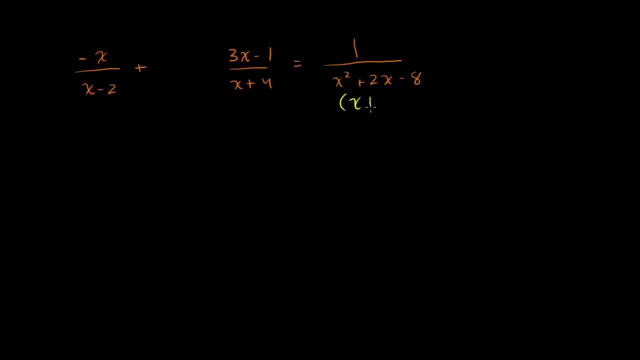 This is: This is x plus 4 times x minus 2.. So it does indeed have both of these in it. So let's multiply both sides of this equation by this thing, or by x plus 4 and x minus 2.. 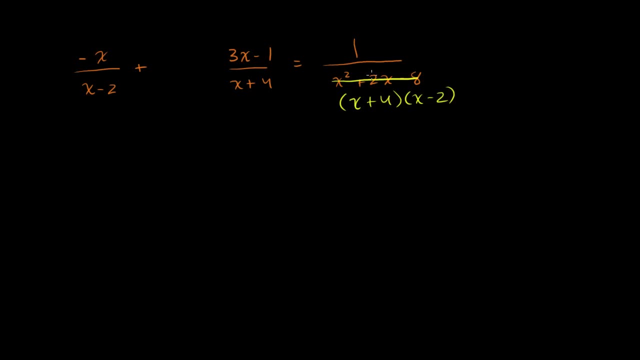 So if we multiply it, So this thing, it can just be rewritten as that. So I just did that. Now let's multiply both sides of this equation by that. So let's see We're going to multiply by x plus 4 times x. 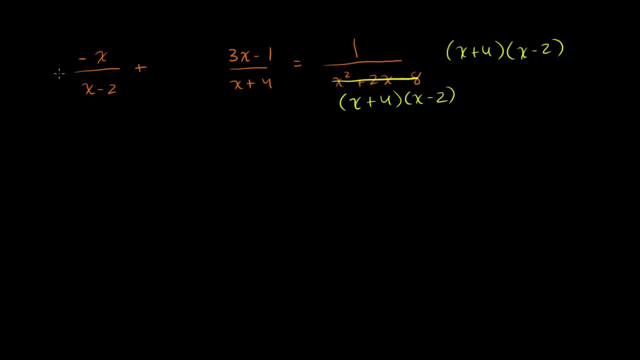 x minus 2.. If we do it on the right-hand side, we have to do it on the left-hand side, Scoot over a little bit. So this term I'm going to have to multiply by x plus 4 times x. 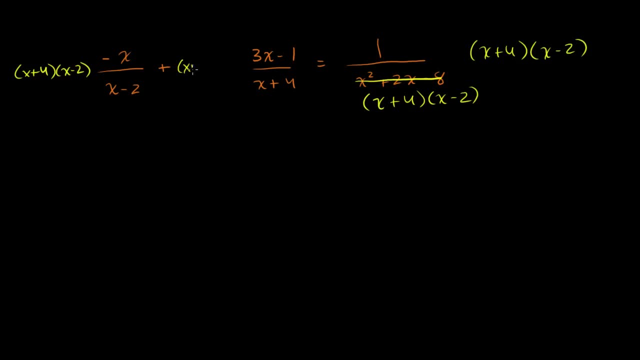 minus 2.. Same thing for this term. That's why I left some space. x plus 4 times x minus 2.. I'm just multiplying every term in this equation by this. right there Now, on the left-hand side, what do we get? 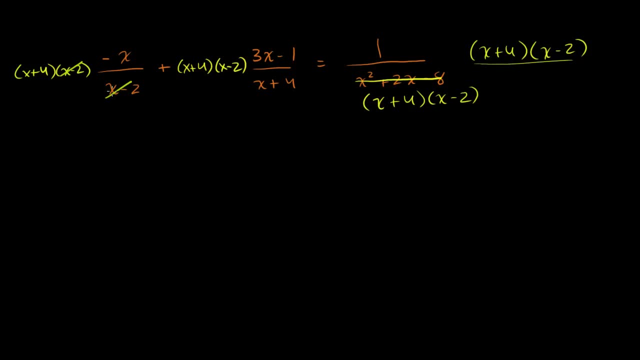 This x minus 2 cancels with this x minus 2.. We have nothing left in the denominator. This term right here will become negative x times x plus 4.. That's that term right there, Now this term and this term right here. 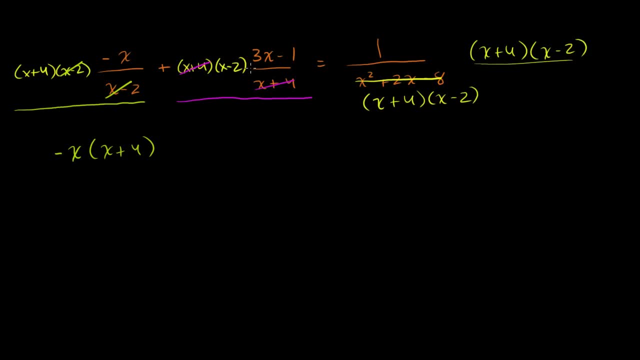 this x plus 4 will cancel with that x plus 4.. So we're left with plus 3x minus 1 times x minus 2.. And then the right-hand side that cancels with that. That cancels with that. 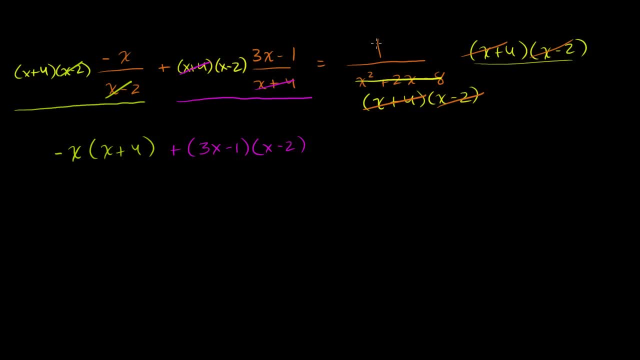 And we've essentially multiplied both sides by this denominator, by the inverse of this whole expression. So we're just left with this 1.. And now we have to simplify it or we have to multiply things out. So negative x times negative x is negative x squared. 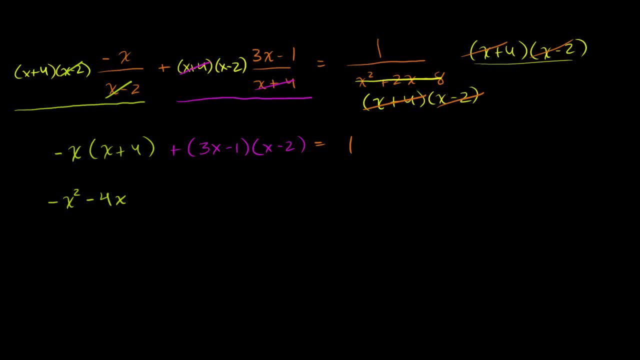 Negative x times 4 is minus 4x. And then we have: 3x times x is plus 3x, squared 3x times negative: 2 is minus 6x. Negative 1 times x is minus 6x. 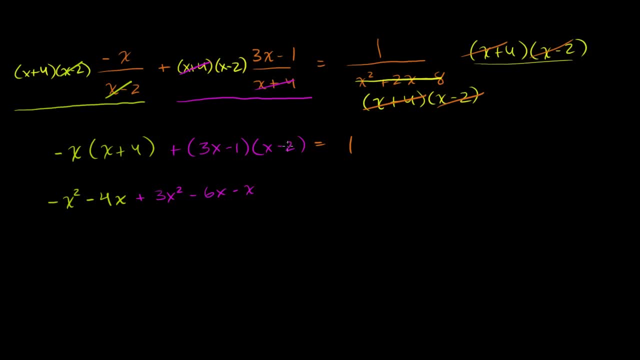 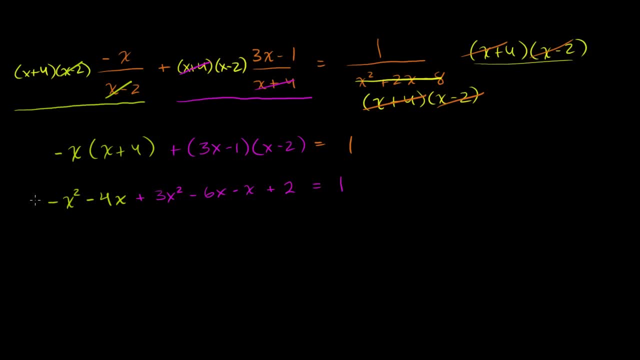 Now let's add the same degree terms. So we have a second degree term and a second degree term 3x squared minus x squared, That gives us 2x squared. Then you have a negative 4x, a negative 6x and a negative x. 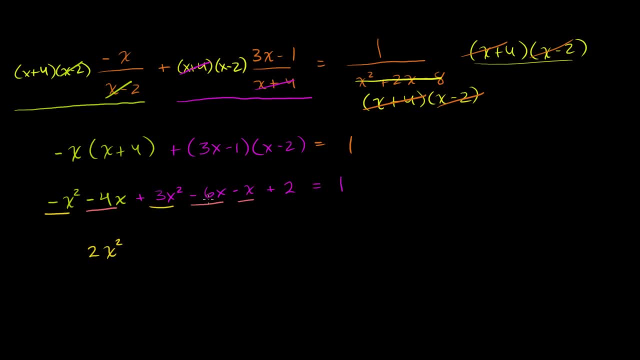 So what is that going to be equal to Negative 4 and a negative 6 is negative 10.. Minus another 1 is a negative 11x, Negative 11x, And then finally, we just have that constant term out here. 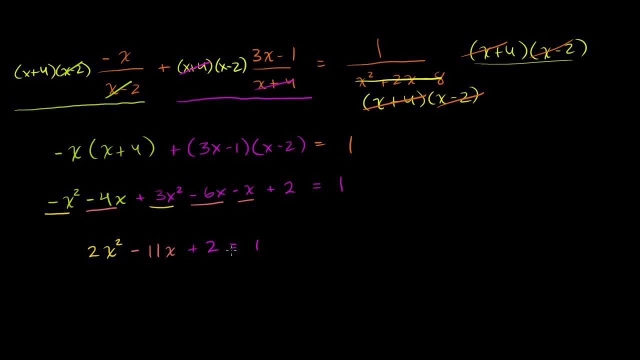 Plus 2 is equal to 1.. And let me make sure, I got all the terms. Yeah, I got all the terms. Now we could subtract 1 from both sides And the equation becomes: 2x squared minus 11x plus 1 is. 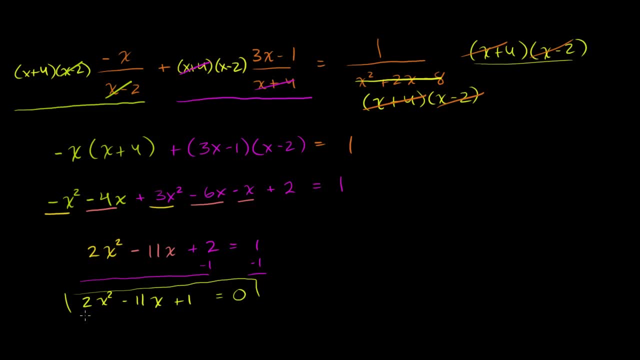 equal to 0.. So it just becomes a straight up traditional quadratic equation And if we're just looking for the roots, we set it equal to 0, we're just looking for the x's that satisfy this, we can use the quadratic formula. 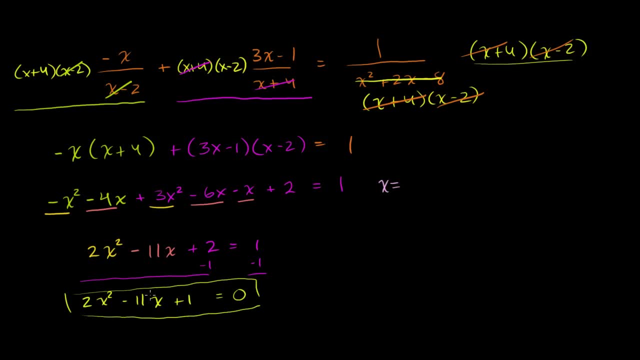 So the solutions are: x is going to be equal to negative b, b is negative 11.. So negative negative 11 is positive 11.. Plus or minus, the square root of b squared, Negative 11 squared, is 121.. Minus 4x. 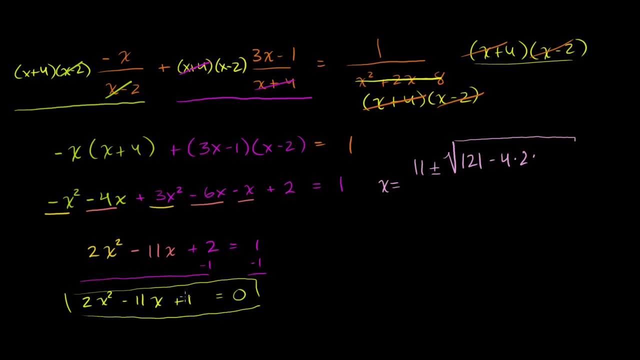 4 times a, which is 2.. Times c, which is 1.. All of that over 2 times a, All of that over 4.. So x is equal to 11 plus or minus. the square root of 4 times 2 times 1 is 8.. 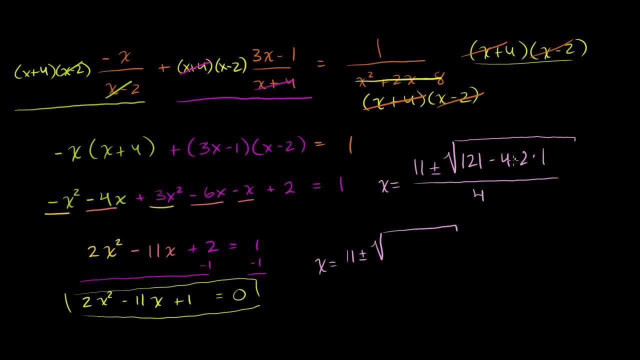 So 121 minus 8.. So what is that? That's 113.. Is that right Square root of 113. And 121 minus 121.. Is that right, All of that over 4.. I don't know, Can I factor 113 at all? 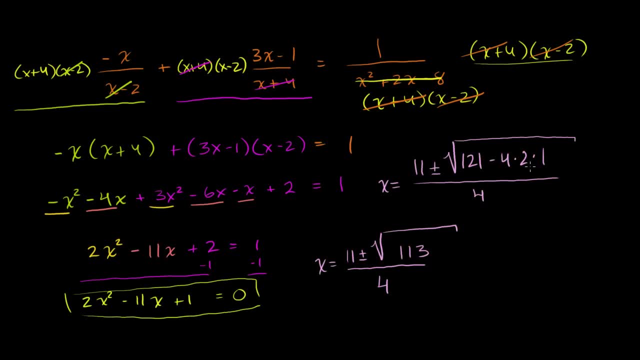 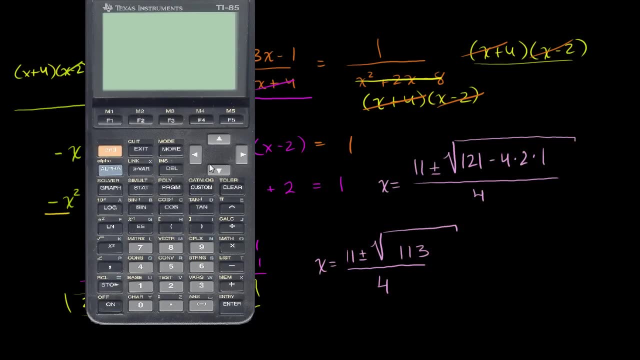 Did I get that right? 4 times, 2 times 1.. Yeah, that looks right. So let's get our calculator out to actually figure out what these values are. Let me see. So we want to turn the calculator on, So go to the Mean screen. 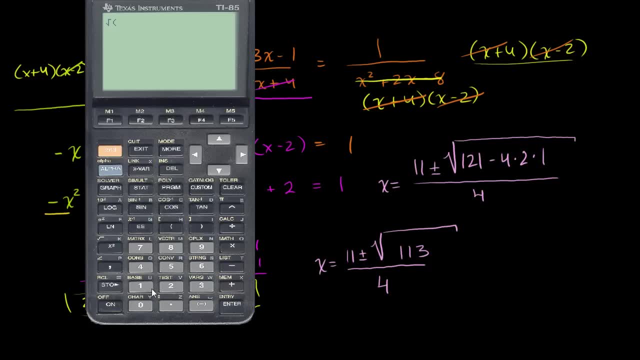 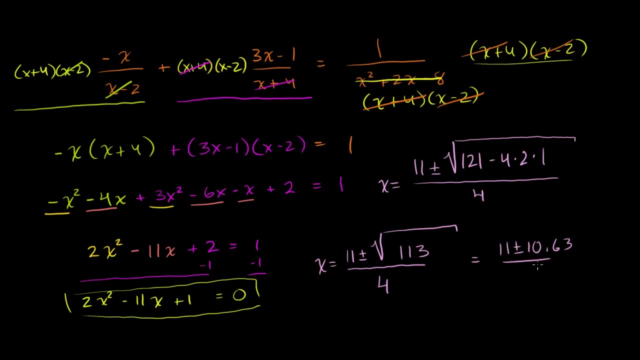 And we want the square root, The square root of 121.. And we want the square root of 121 minus 8.. So this is equal to 11 plus or minus 10.63 over 4.. Those are our two answers. 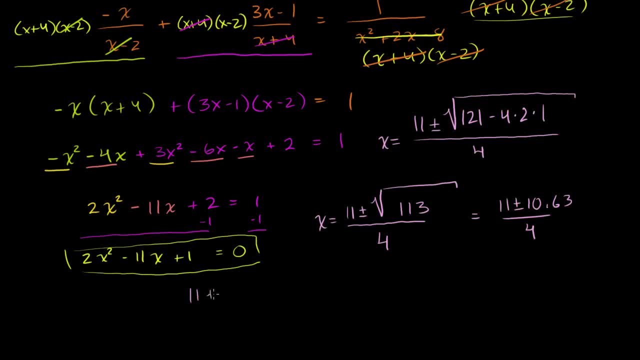 And if we want to find the particular answers, it would be 11 plus 10.63 over 4, which would be what? That would be, 21.63 over 4.. We could try to calculate that in a second And then, if you subtract it, 11 minus 10.63 is 11 minus 10.63. 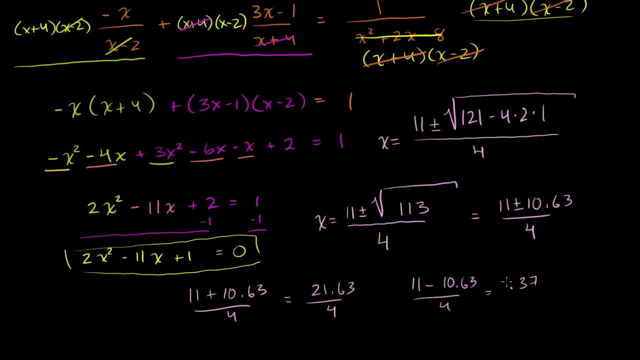 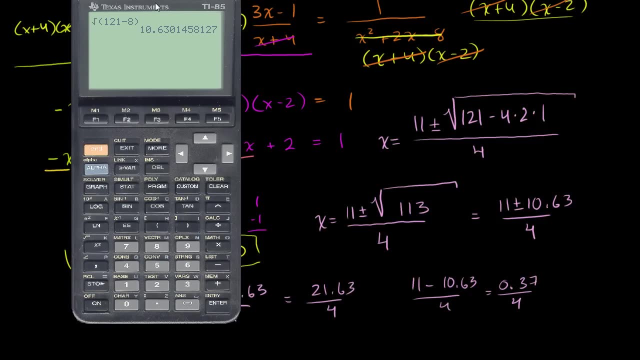 over 4.. This is equal to what Like 0.37.. 0.37 over 4, if I'm doing my math correctly. So what do we get? So let's see: 21.63 divided by 4 is 5.41.. 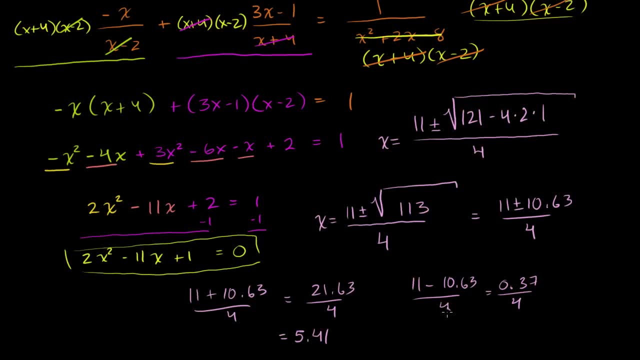 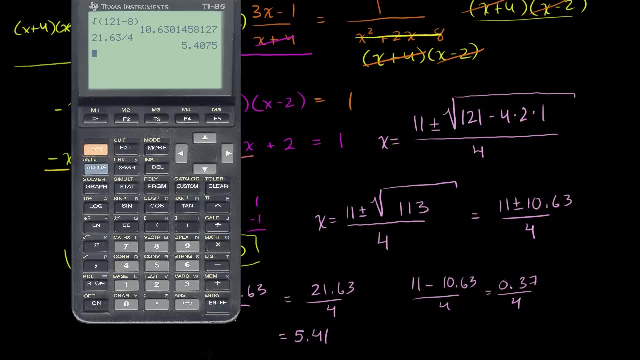 So this is equal to 11 minus 10.63 over 4.. This is equal to 5.41.. And then the other solution, 0.37 divided by 4, is going to be like 0.09 something. 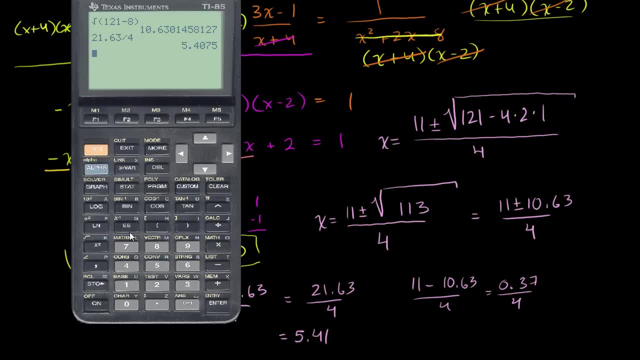 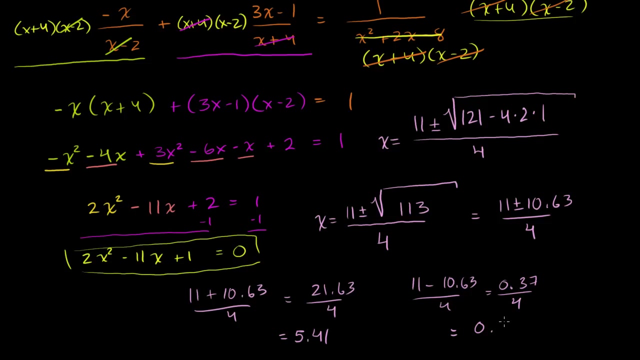 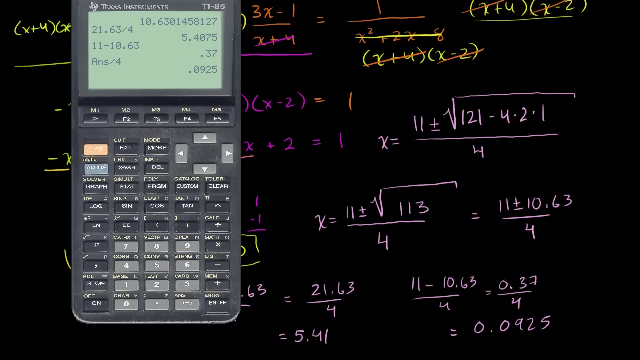 So then we have: the other solution is 11 minus 10.63.. Yep, we got our: 0.37 divided by 4 is equal to 0.0925.. So this is equal to 0.0925.. So I lost some precision. 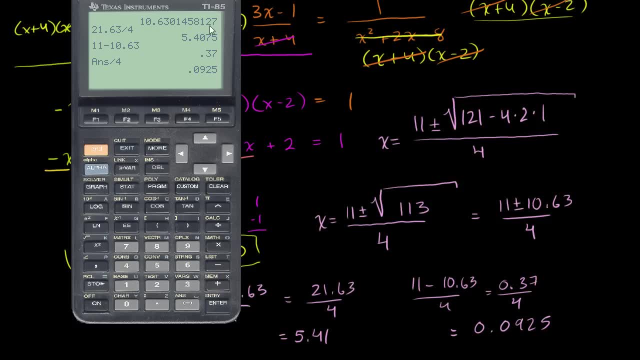 This isn't the exact, because this wasn't 10.63,, it was 6301.. It just kept going. It's an irrational number, But this should get close. So let's check, Let's verify that these actually work. 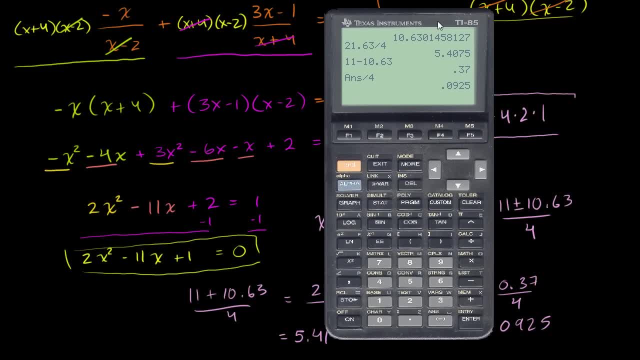 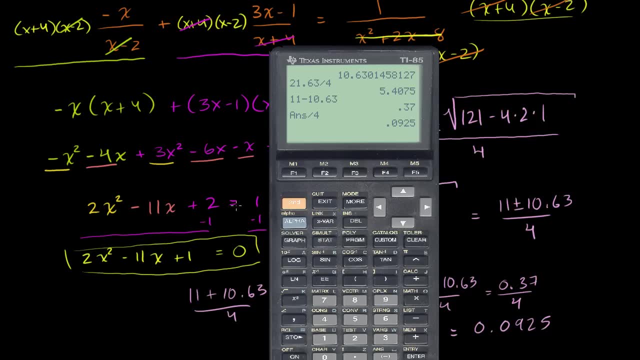 So let's try the 5.41 solution first. So if this is true, If this is true, If we take: So let me put 5.41,. well, let me just do it. So if we do so, we're going to start off with 5.41.. 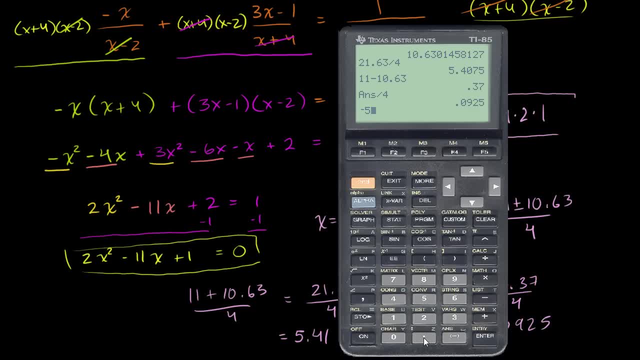 So our original equation was negative x, So negative 5.41 divided by x minus 2.. So 5.41 minus 2 is 3.41.. So that's that term, And then we have plus 3 times 5.41.. 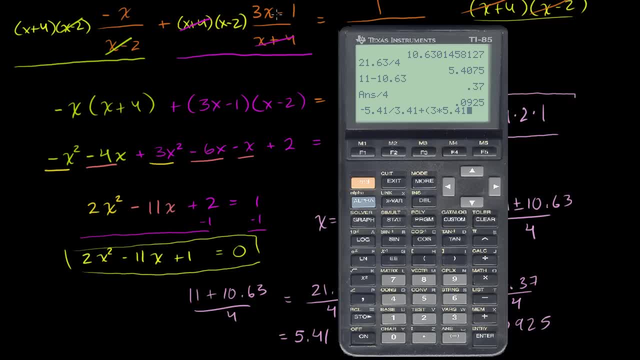 So that's that term. And then we have plus 3 times 5.41.. So that's that term. And then we have plus 3 times 5.41, minus 1. divided by 5.41 plus 4 is 9.41.. 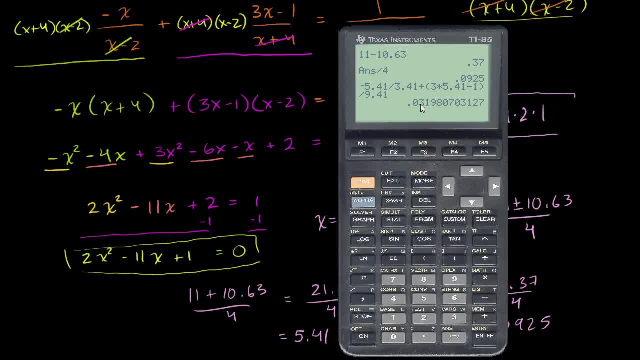 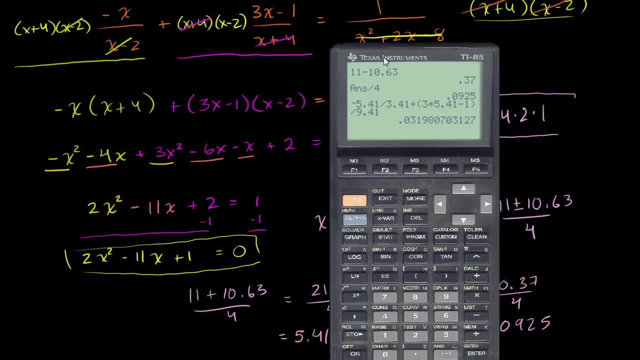 So the left-hand side gives us 0.0319.. So that's what the left-hand side equals. And let's see what the right-hand side equals. when we substitute x equal 5.41.. And of course we've lost some precision here. 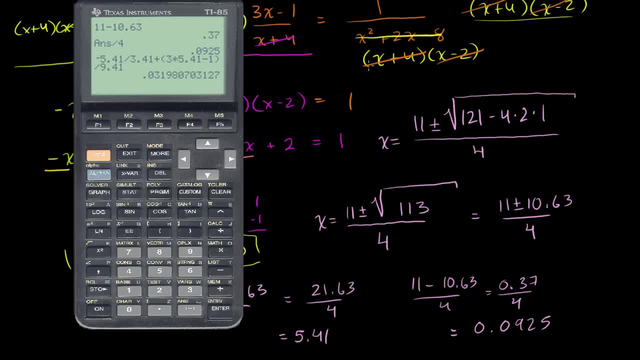 We've lost some of the 0's, but we should get pretty close. So the right-hand side, if we take 1 divided by 5.41, squared plus 2 times 5.41 plus this is a minus 8, I think. 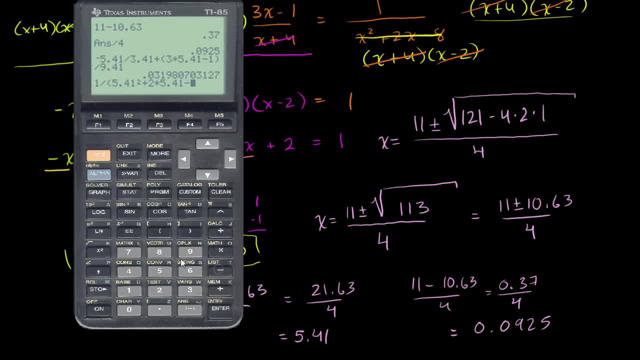